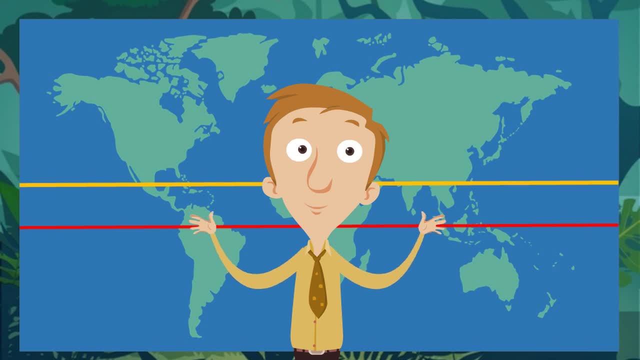 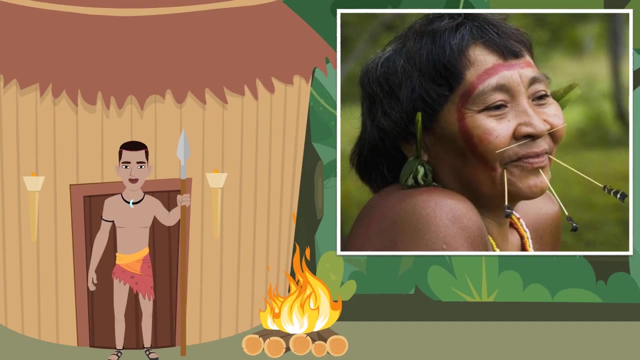 Today we're going to head back into the Amazon to meet a tribe of people who were very much unknown to the rest of the world until very recently. Let's go meet the Yanomami tribe of the Amazon. The Yanomami tribe is one of the largest tribes of people who live. 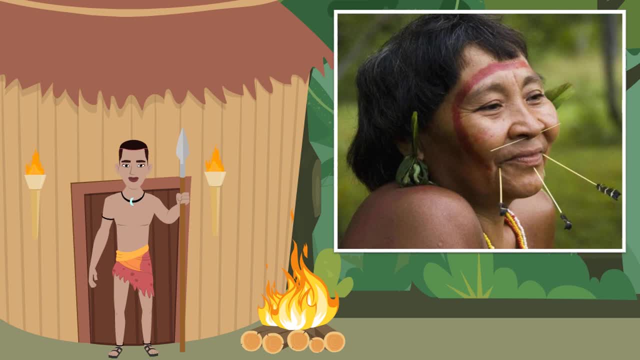 in the Amazon rainforest. They live deep in the rainforest, far away from any modern cities or towns. In fact, the rest of the world didn't even know that they existed. until the 1960s, The Yanomami tribe had been living completely isolated away from the rest of the world. 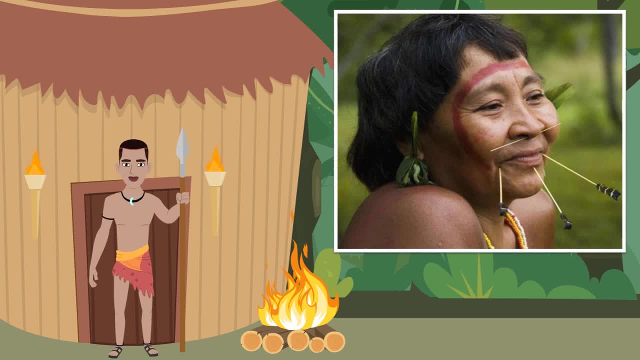 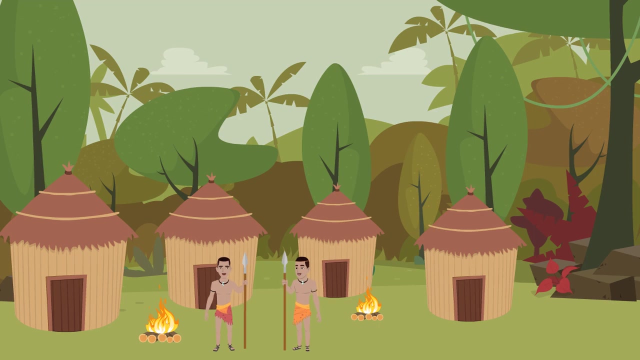 And they continued to live a life in a very traditional way. What do you imagine the Yanomami villages to look like? Pause the video and draw a quick little sketch of what you think their houses would look like. Well, the Yanomami live in small villages in the rainforest. Each family has got a shabono. 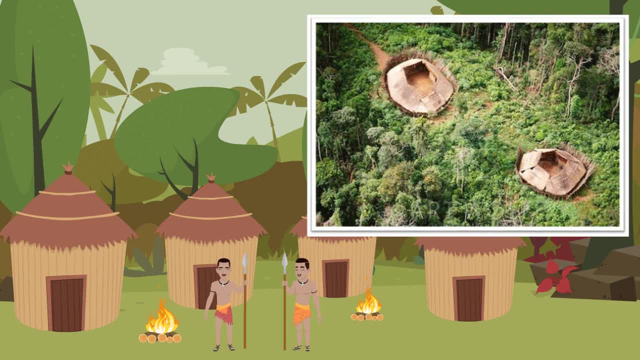 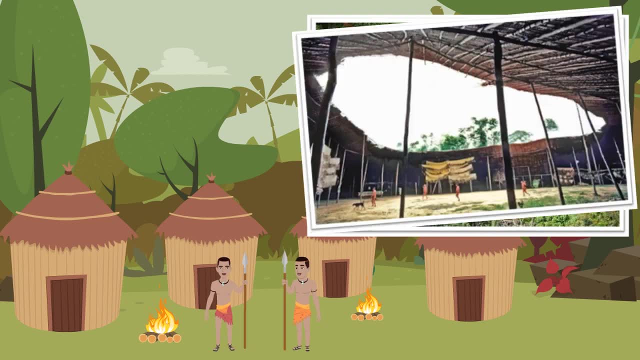 which is a large hut With a space in the middle. The whole family lives there. The shabonos are made in clear patches of ground in the rainforest. They're made out of palm leaves and wood from the area around And they can be pretty long- As long as 100 meters, Kind of like a rainforest. 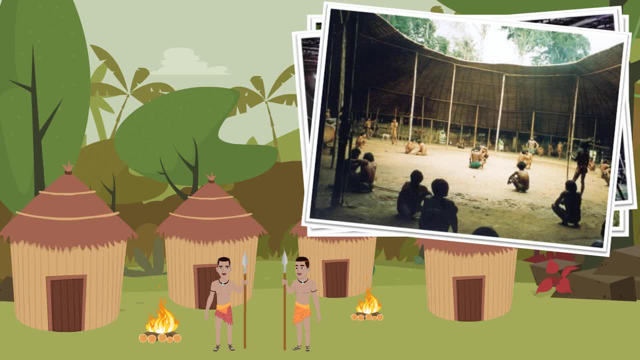 mansion. These houses, though, are not forever. Every few years, they break down the shabono and build a brand new one out of new material. That's quite different to how we build houses where we live. Can you imagine if, every few years, you had to knock down your home and rebuild it again from just the stuff you can gather? 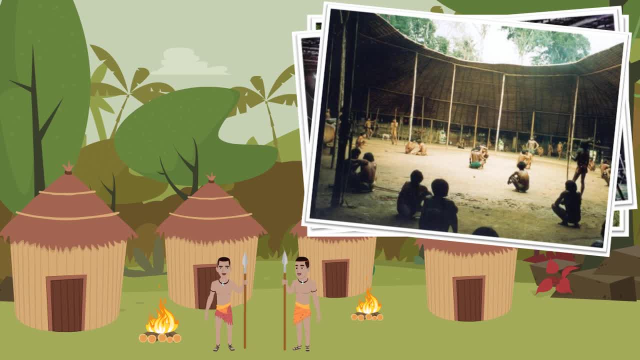 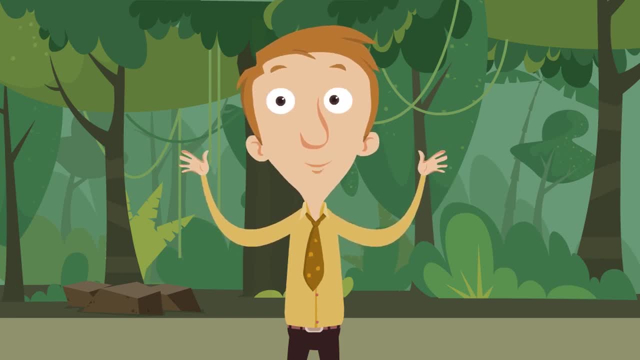 It would be very difficult to do that in Dublin city. What about the food that the Yanomami eat? What kind of things do you think they would be eating in the rainforest? Pause the video and write down two things that you think they would be eating in the rainforest. Pause the video and write down two. 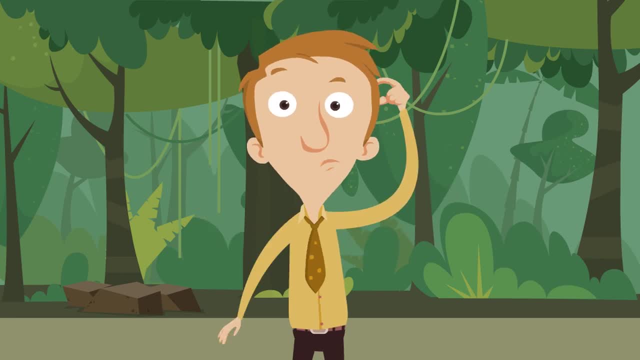 two things that you think they would be eating in the rainforest. Pause the video and write down two, two foods you think they might eat. Well, as you can imagine, in the middle of the Amazon rainforest there is no McDonald's. there is. 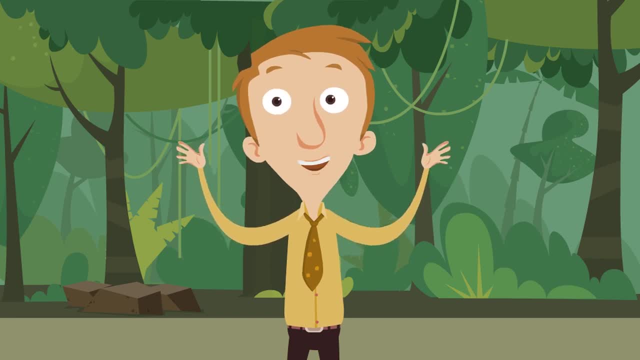 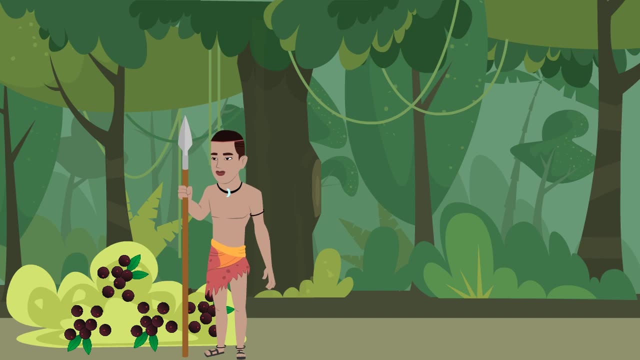 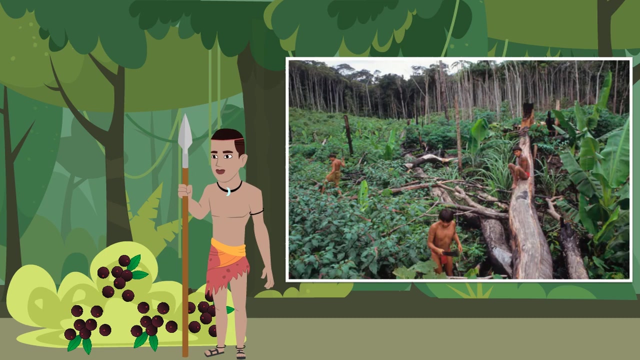 no KFC and there is no Tesco. The Yanomami tribe have to get all their food from hunting, fishing and growing crops. The men clear sections of the jungle, so the women can plant fruit and vegetables like bananas and sweet. 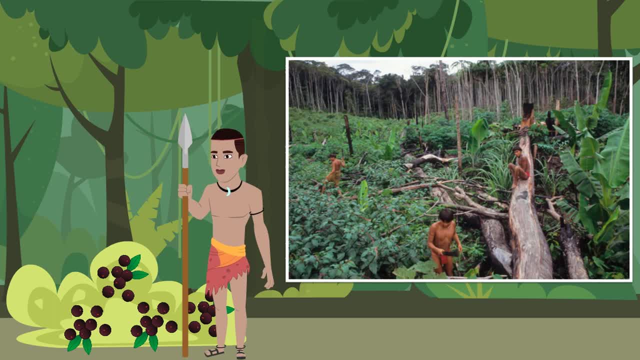 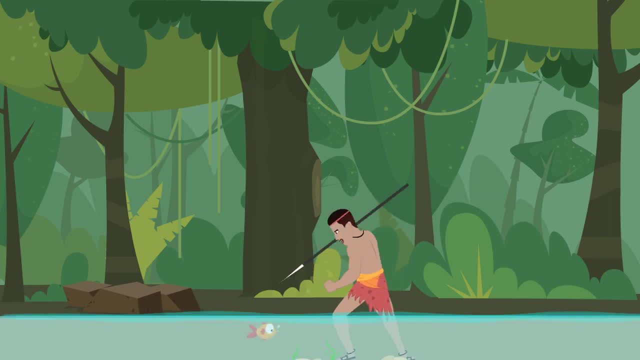 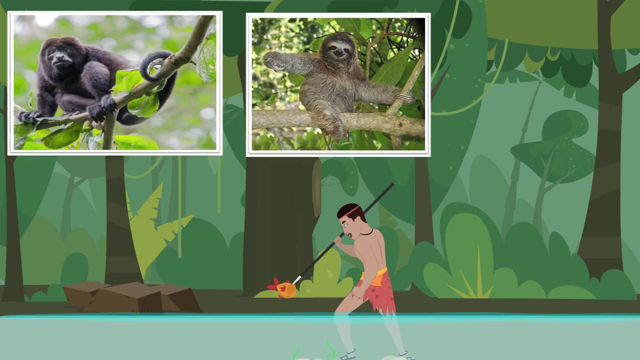 potatoes. They also gather fruit and berry from the rainforest. The men have the job of hunting animals, and the animals they eat might surprise you. They hunt things like monkeys, sloths, birds and pumas, as well as fish. They use. 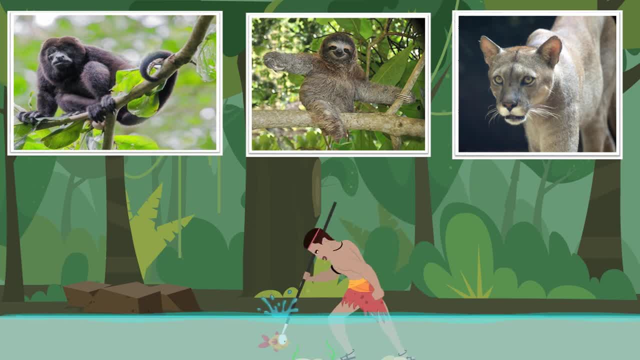 poison darts to kill their prey. You've heard about these poison darts before in a science lesson. Can you remember where they get the poison from? Pause the video and write down the answer. Well, if you remember from the science lesson the other day, 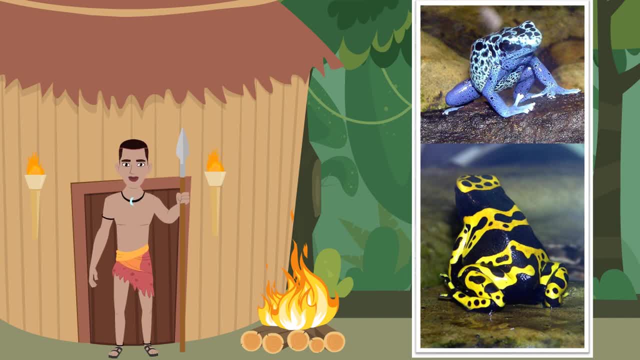 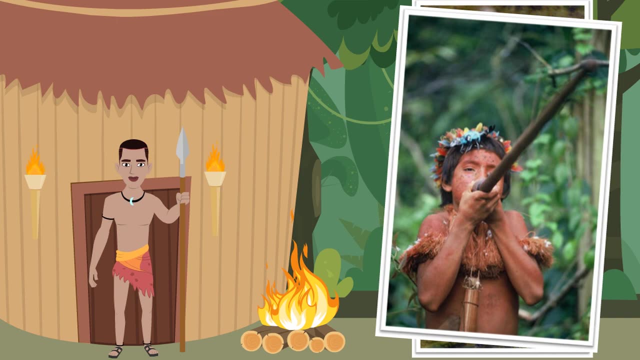 these poison darts are made using the poison taken from the poison dart frog. The hunters use bow and arrows to hunt their prey, but they also use- some of them use- a special piece of equipment called a blowpipe. This is a hollow tube that 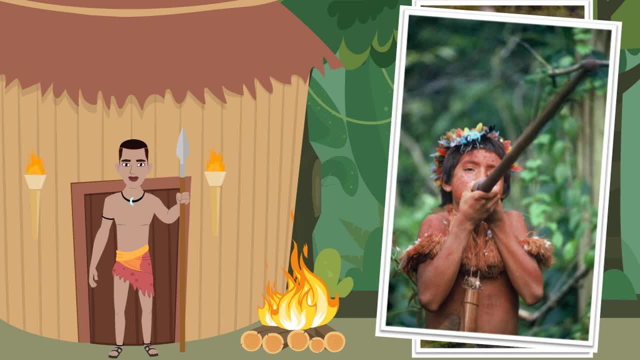 the dart is placed in, and you blow really hard on one end to shoot the dart out. You have to be careful, though. If you swallow the poison dart, you are in big trouble, because there's no hospitals in the rainforest. What about the children in the village, though? 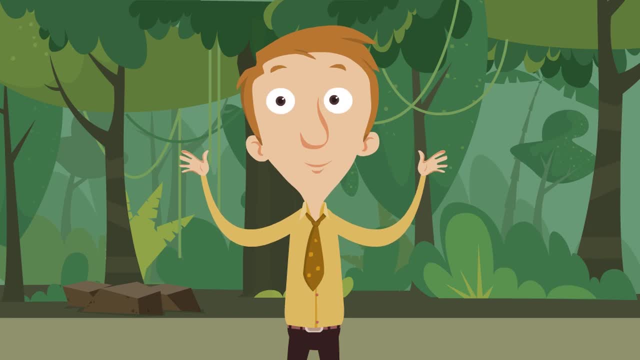 What do you think they do all day? Do they go to school like you Or do they do something different? Pause the video and write down what you think they might do. Well, the boys and the girls in the village live two very different. 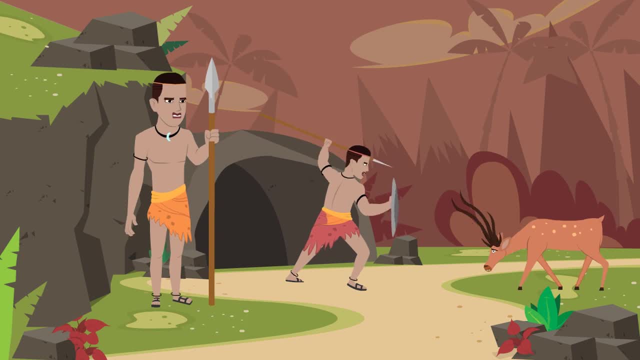 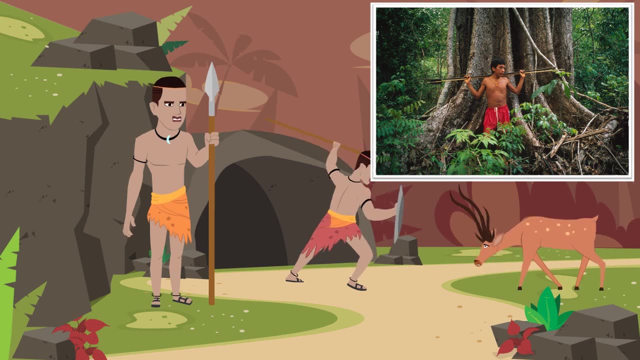 different lives. The boys learn to hunt from a young age so that when they grow up they'll be able to provide for their family. Sometimes they go out with the men for days on end learning how to hunt and track animals. 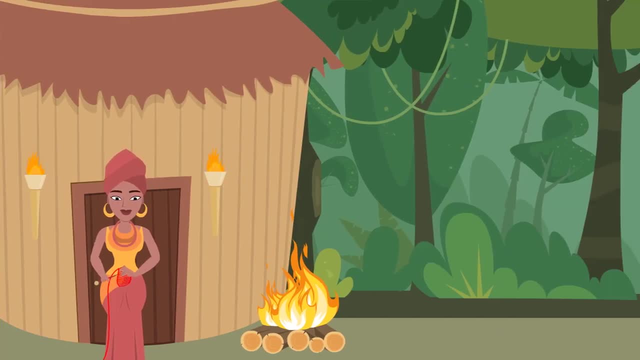 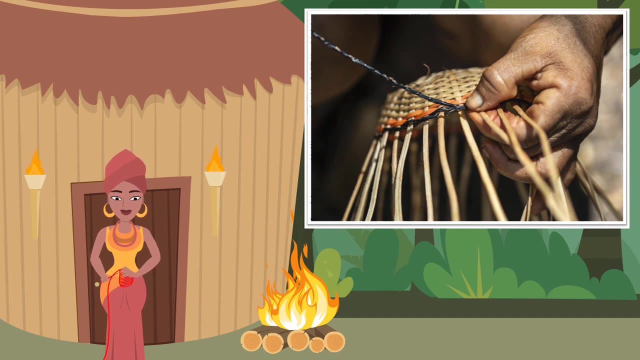 The girls stay at home with their mothers until they get married and learn to gather and prepare food. They also look for vines that can be woven into baskets and other tools. But what do the Yanomami tribes do for fun, Do they? 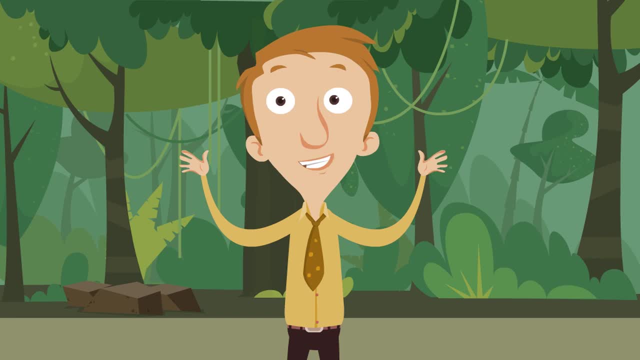 play sports like football? Do they jump onto their playstations and play some Fortnite? Pause the video and write down what you think they might do for fun. Well, of course, there's no Xboxes or playstations out in the rainforest. 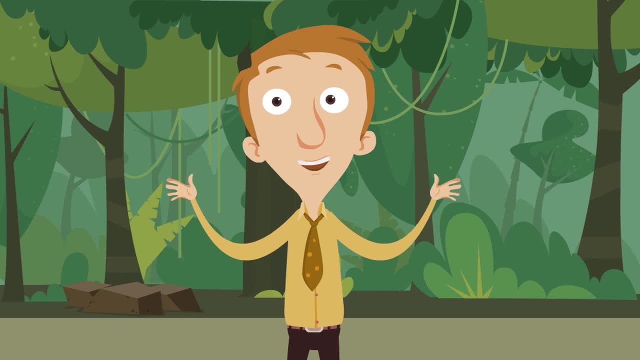 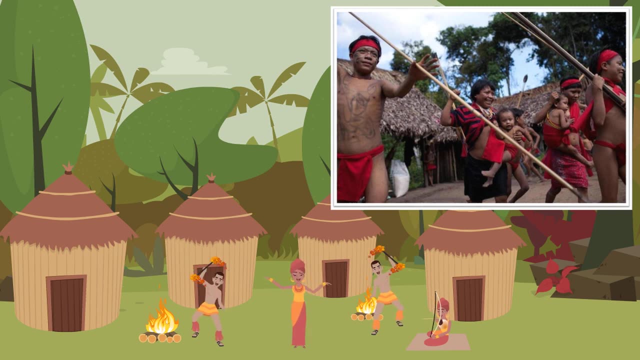 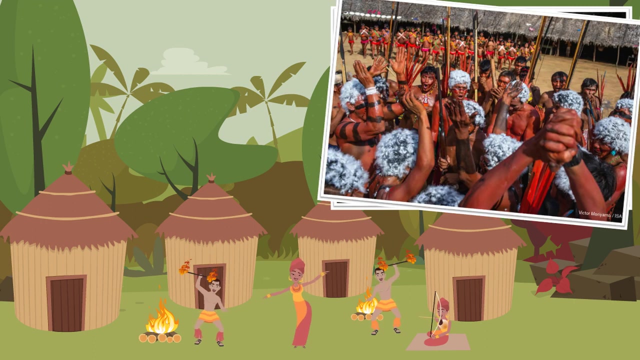 so the Yanomami tribes find a different way of having fun. They celebrate special events with massive feasts, They invite all the neighboring villages to join in and they have lots of food, music and plenty of dancing. They decorate their bodies with paint and they decorate. 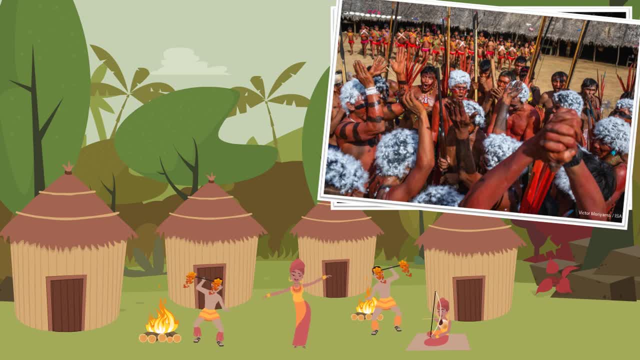 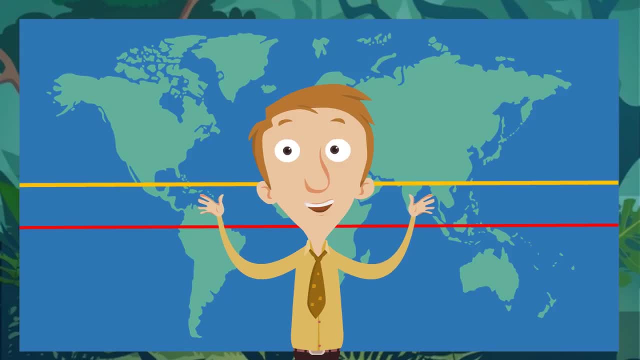 their faces by placing small sticks through their nose and chin, like in the picture on the side. The Yanomami tribe are only one group of people who live in the rainforest. There are lots of other tribes like the Yanomami who live. 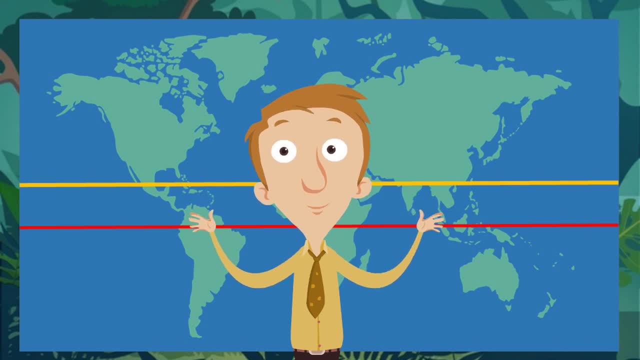 in all of our other rainforests. Have a look at the pictures on the next few slides. What can you learn about the lives of the traditional tribal people from the pictures that you're seeing? Let's have a look at the first one. 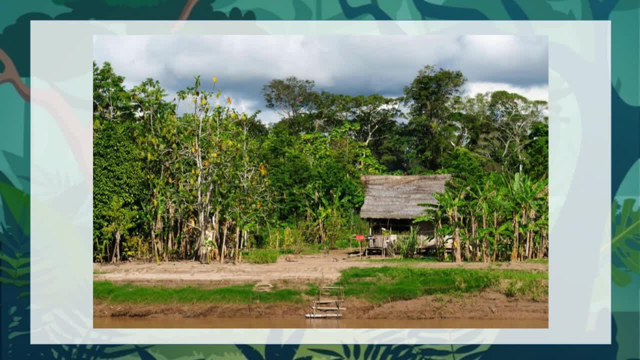 In this picture we can see the type of housing that the people in the rainforest build. You can see the materials that they use and you can see what's around them. Pause the video and write down one thing that's the same and one thing. 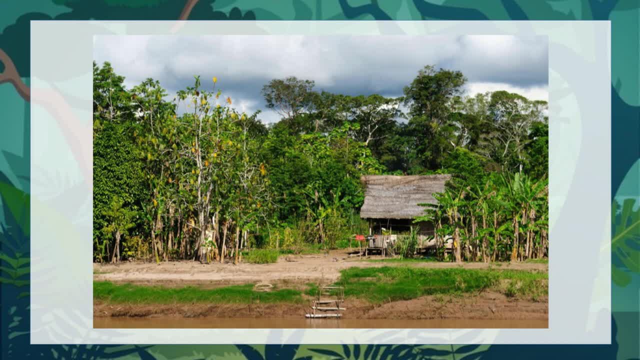 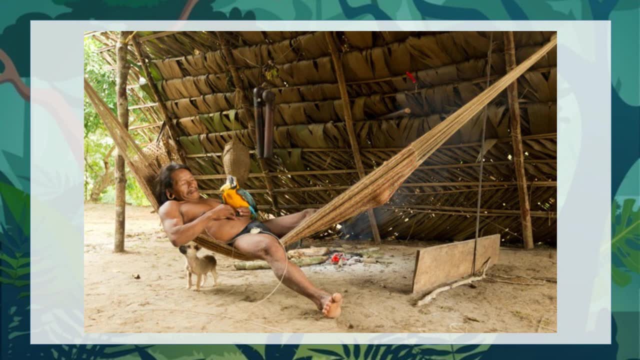 that's different Between this home and your home. Let's look at another picture. Ah, take a look at this tribal man relaxing in his bedroom with his pets. Pause the video and write down. one thing that's the same and one thing that's different. 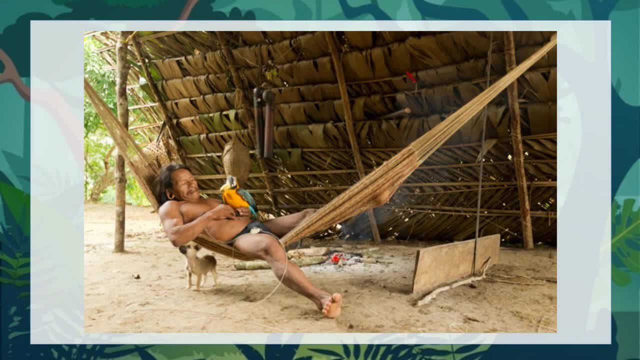 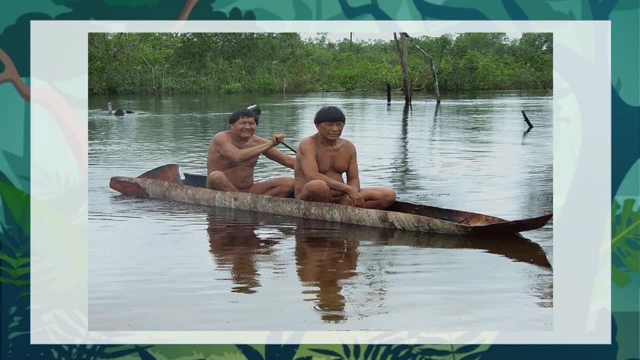 Between relaxing in your bedroom in the rainforest and relaxing in the bedroom in your home. Take a look at another picture. Ah, here's the two gentlemen out for the day, probably traveling to somewhere a little bit far away, Maybe public transport. Pause the video. 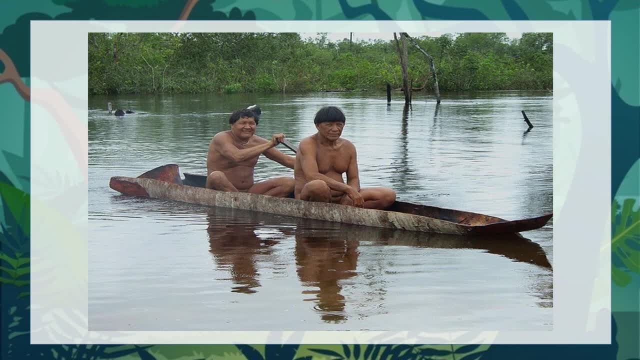 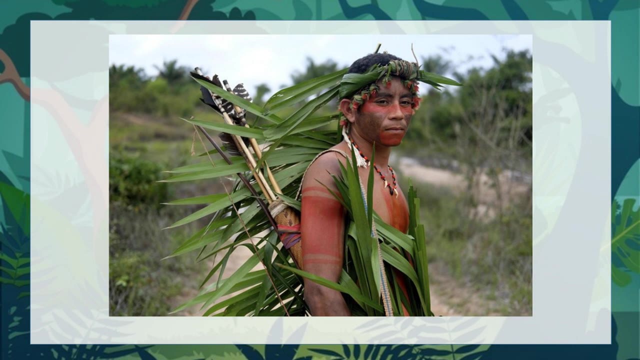 and write down one thing that's the same and one thing that's different about traveling in the rainforest and traveling places in town. Let's have a look at one more picture. Here we can see a tribal man going out to get the dinner.